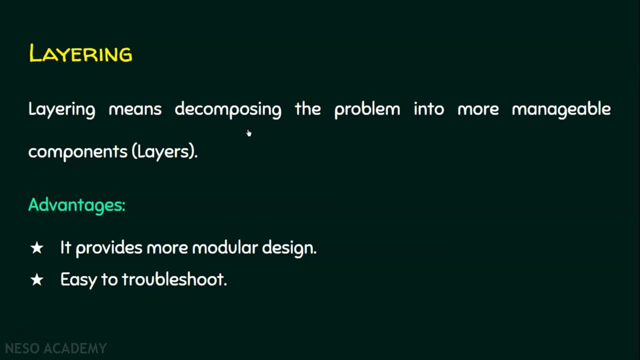 For example, if we are supposed to solve a big problem, instead of solving a big problem at once, we can break that big problem into smaller problems if we solve all smaller problems and obviously the big problem is solved. So layering means decomposing the problem. 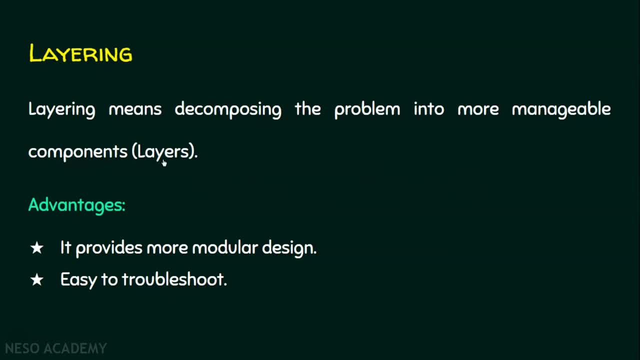 into more manageable components or layers, which has two advantages: It provides more modular design. In computer science we know very well that modularity has its own advantages, Where big problem is broken into smaller problems and we are able to solve smaller problems effectively. 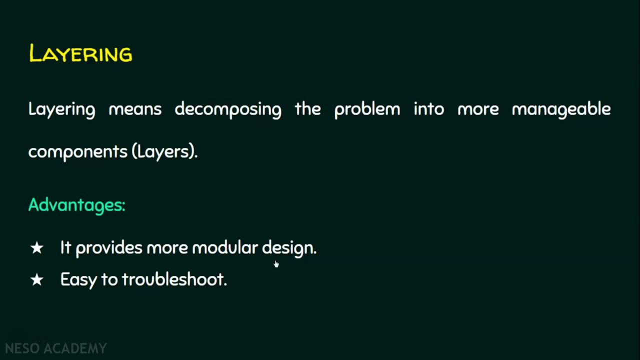 so that we can get the solution for the big problem. Likewise in computer networking also we are going to use such kind of modular design And also it is easy to troubleshoot. Suppose if we have five layers and there is a problem. 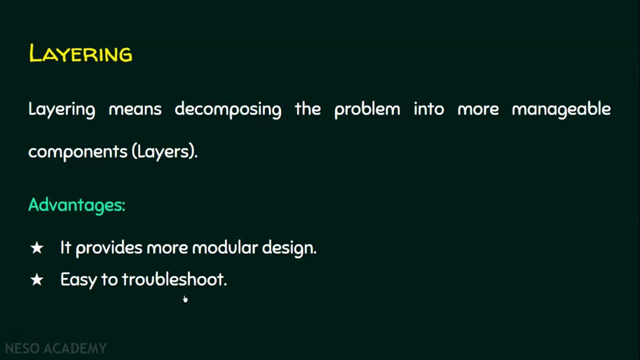 in one layer. we need not go and check other layers, We can just focus on the layer which has encountered an error. So that's the power of layering. It provides more modular design and it is easy to troubleshoot. So far we have seen what is layering. 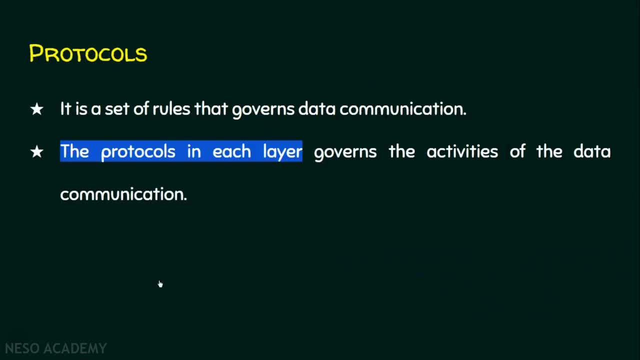 Now we will see what is the role of protocols in layering. We know very well that protocols is a set of rules that governs data communication And the protocols in each layer governs the activities of data communication. We have seen in the previous lectures that 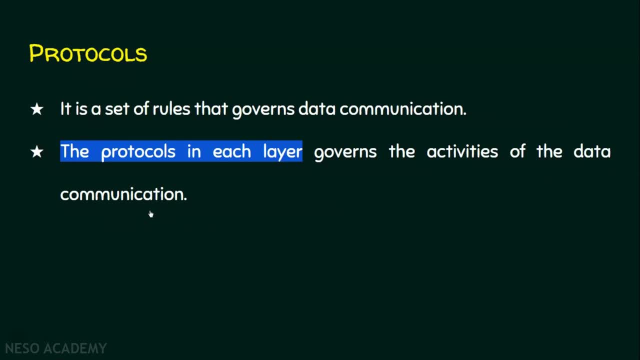 we are going to add IP address, MAC address and port address with data before sending the data. So in each layer we are going to address each of these addressing And each of these addressing are taken care by different protocols. That is what is mentioned here. 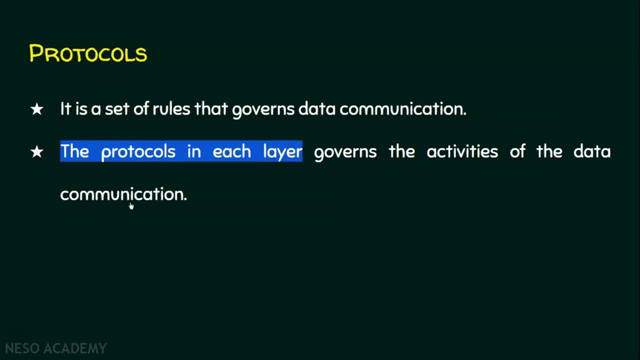 The protocols in each layer governs the activities of the data communication And ultimately we want effective data communication, So we need certain rules to govern this data communication. Which protocols takes care? Now we will see what are the layered architectures available. 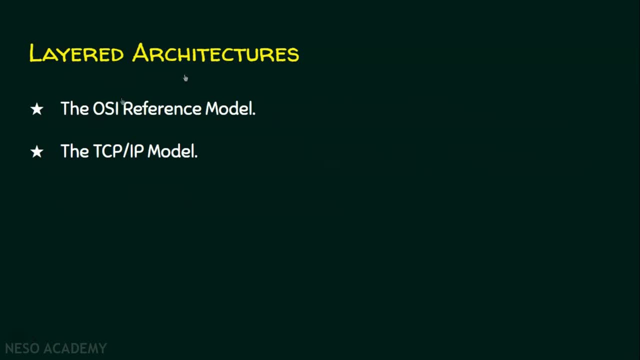 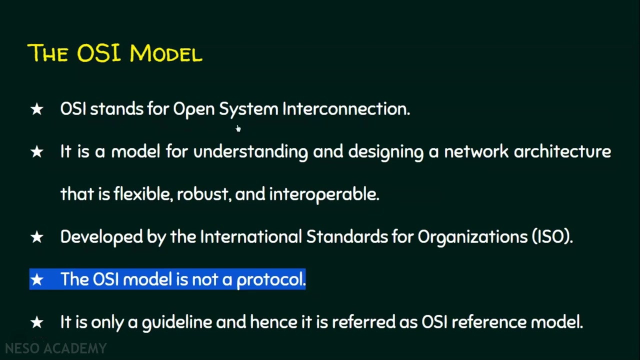 We are going to focus on two layered architectures in this series: Number one, the OSI reference model, and number two, the TCP IP model. We will see the OSI reference model now, The OSI model. OSI stands for Open System Interconnection. It is a model for understanding and designing a network architecture. 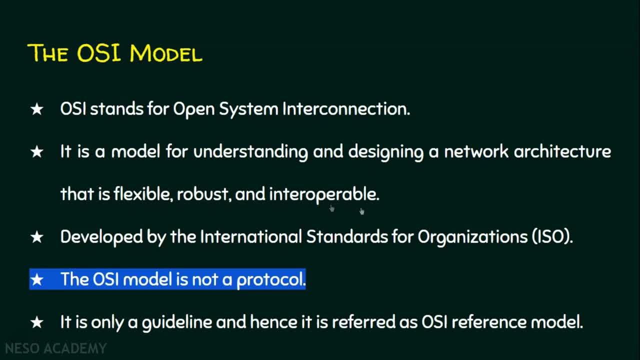 that is flexible, robust and interoperable. If you don't understand this, just listen to this example. Suppose there are two computers And we are intended to have communication between these two computers, And so obviously we are going to form a network. 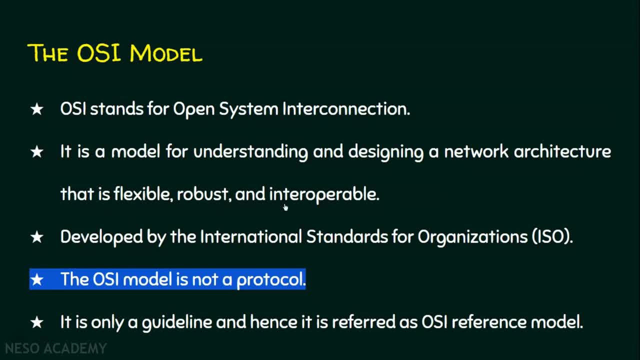 This network architecture should be flexible, robust and interoperable. Interoperable means, suppose, if one computer is sending data which is generated by Windows operating system and that should be acceptable by other computer in Linux operating system. So that is what is interoperable. 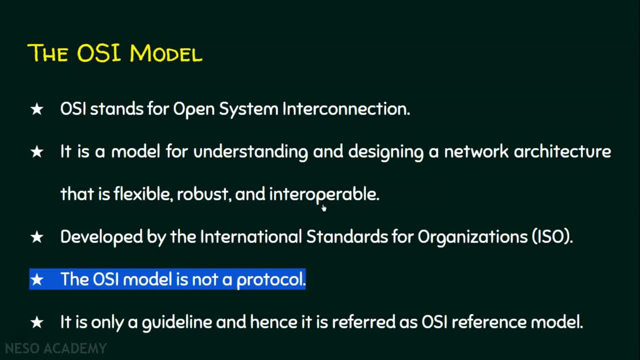 And not only in terms of operating system, in terms of applications too. This network architecture should be robust- We should rely upon this communication- and it should be flexible enough too. This OSI model is developed by the International Standards for Organizations, which is well known with this acronym ISO. 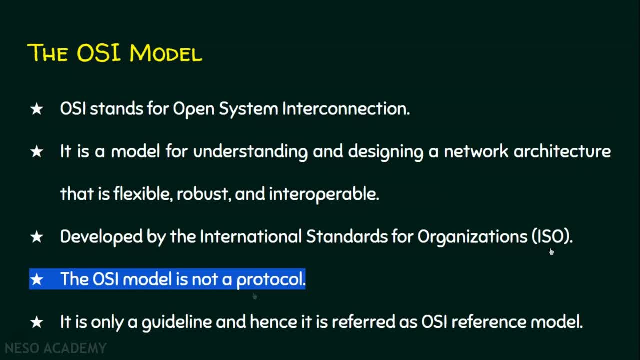 So ISO developed this OSI model. The very important note is that the OSI model is not a protocol, So it is not implemented. It is only a guideline for two different computers or two different systems wants to communicate with each other. They can follow these guidelines. 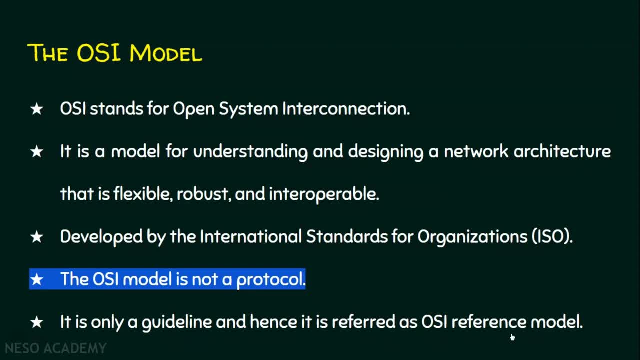 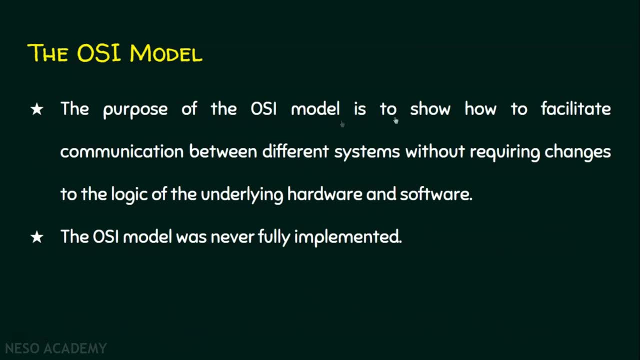 And hence it is referred as the OSI reference model. We will now see what is the purpose of having this OSI model. The purpose of the OSI model is to show how to facilitate communication between different systems without requiring changes to the logic of the underlying hardware and software. 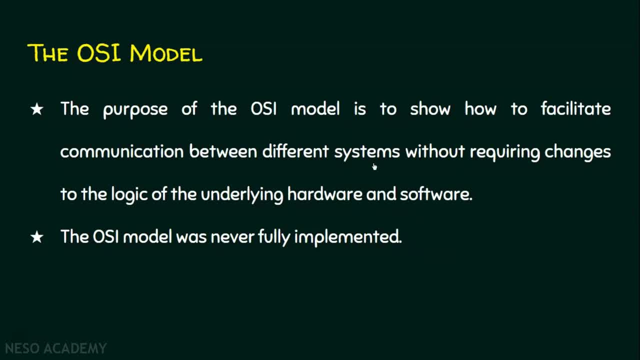 If it is very lengthy, just listen to this. If there are two different systems, that wants to communicate with each other. So we want to establish communication between two different systems: One system which is running with Windows operating system and another system is running with Linux operating system. 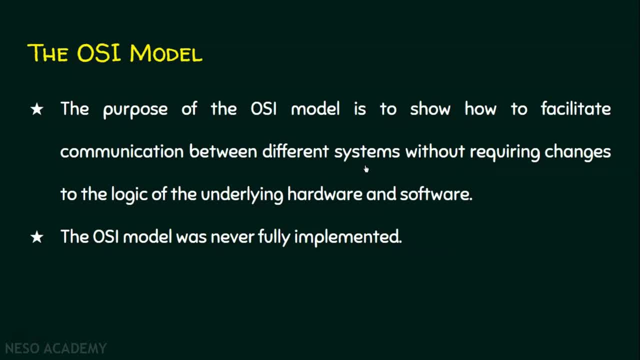 But our protocols should convert the data in such a way that any operating system should understand that data. So that is what is mentioned. So the communication between different systems should be facilitated without requiring changes to the logic of the underlying hardware and software. 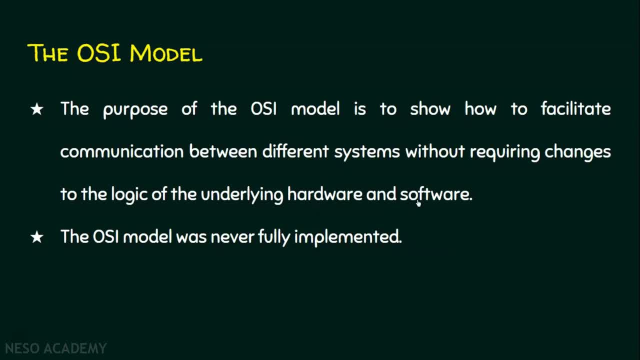 without requiring changes to the logic of the underlying hardware and software. If two different architectures- one is using Motorola architecture, another one is using Intel architecture- it should not be a problem for computer communication. So, irrespective of hardware and software, the computer communication should happen between different systems.